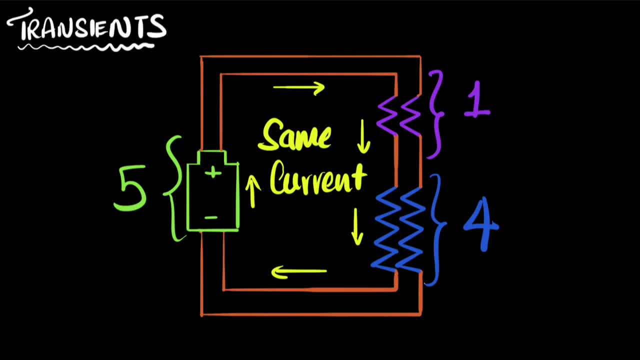 milliseconds. we give it a name. We call it the transient stage or the transience. So let's look at the transient stage in this entire entire video. So we've just closed the switch, We have closed our circuit And let's slow down. 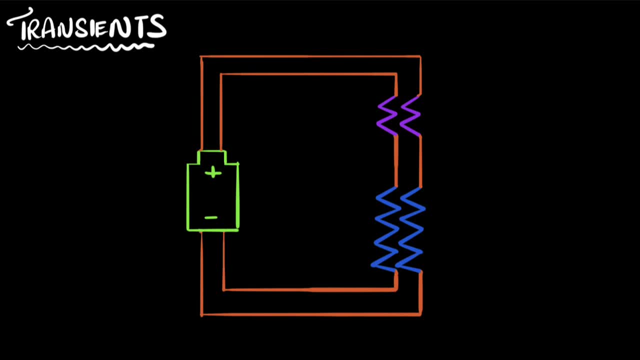 time. What's going to happen? Well, we have electrons everywhere And these electrons have not yet started moving. We have yet to have a current, We've yet to have a voltage. What's going to happen to these electrons? Well, the battery is going to start pulling and pushing. 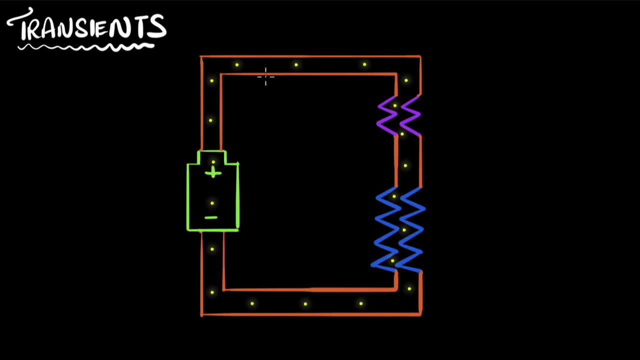 on them. The negative charge is going to push on the electrons, The positive charge is going to pull on the electrons, So there'll be a force that every single electron will feel due to the battery. And all these forces are pretty much the same. 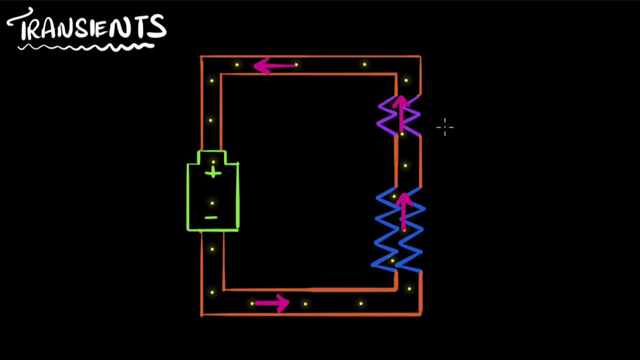 right now, The battery is not conspiring to do anything. The battery doesn't care where the resistors are. The forces are the same. What's going to happen because of that? Well, now the electrons will start moving and we're going to have a current. If you look at this section of 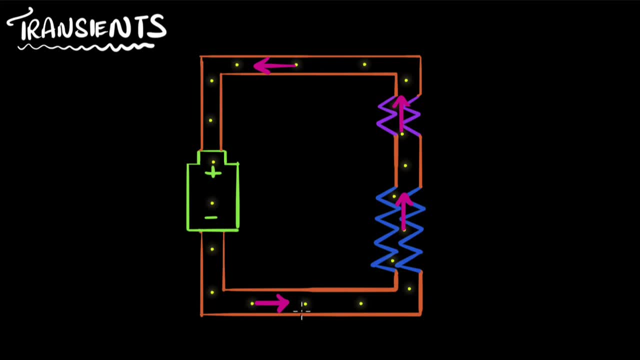 the wire with no resistance, the electrons are going to go very, very high speed And therefore we're going to have very, very high current. So we'll have huge current in these sections of the wire which have no resistance. I'm going to draw thick wires, thick lines of 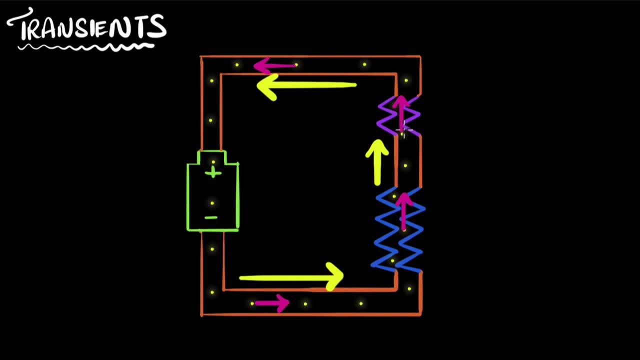 current for that? What about this section of the wire which has some resistance? Well, electrons are going to go a little slower, They're going to find it a little harder to go And therefore the current over here will be smaller. And I'm going to draw a little thinner direction. 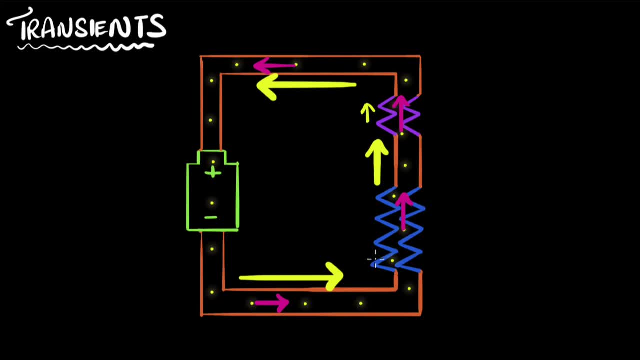 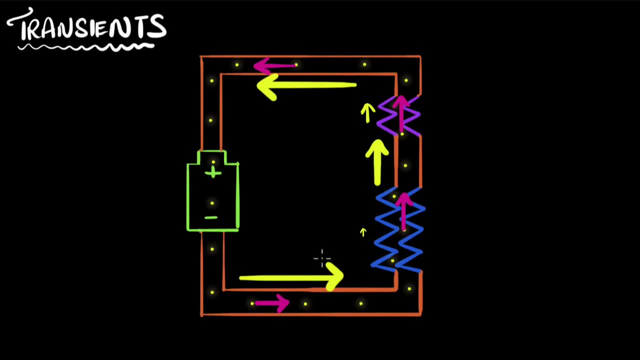 very tiny And at this moment, right in front of your eyes, you can see, in the transient stage, the current is not the same everywhere. This is the stage where the electrons are experiencing the same force as of now, but the current is not the same And eventually, later on, by the time you 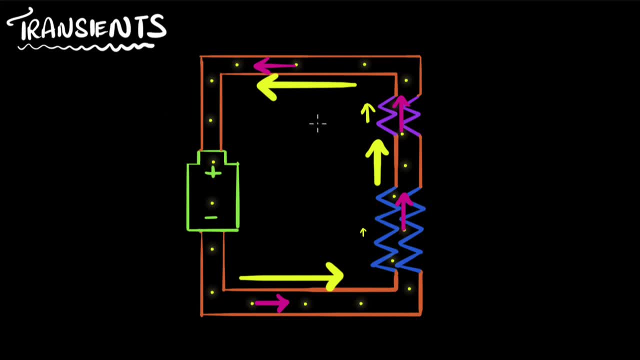 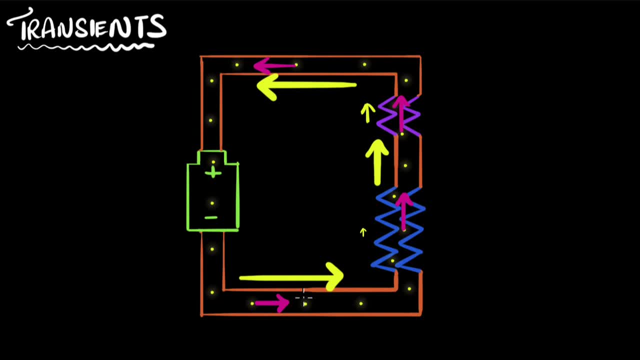 very pretty, And the whole idea is to see how we go from here to there automatically. how does it happen? Okay, To see how that happens, we need to look at the ends of the resistor. That's where things are interesting, because that's where the current changes right. So let's look at the ends. 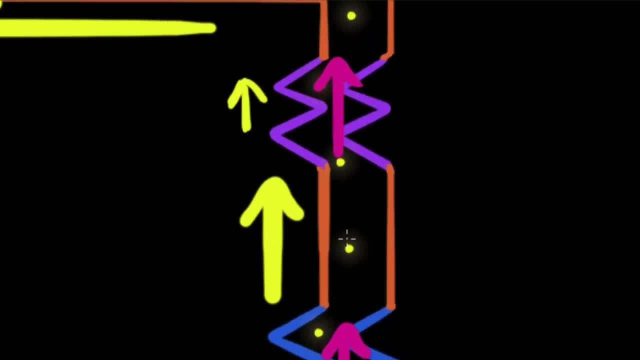 of this resistor. If I focus on this end, you can see electrons are coming in at very high speeds. A lot of electrons will be coming in per second, but the electron's going out of this point into this resistor will be less per second. So we need to take the electrons inside out from here and 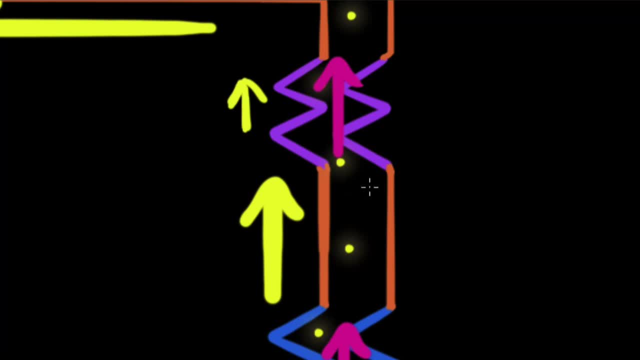 What's gonna happen because of that? Because of that, you will have traffic jam. You'll have electrons getting accumulated over here. Imagine you have 10 electrons coming in per second and only two electrons going out per second. Eight electrons will get accumulated, right? 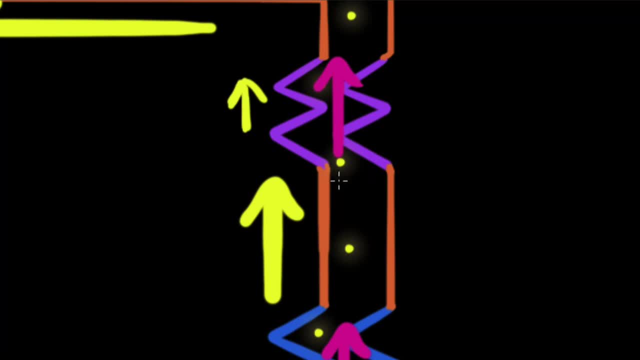 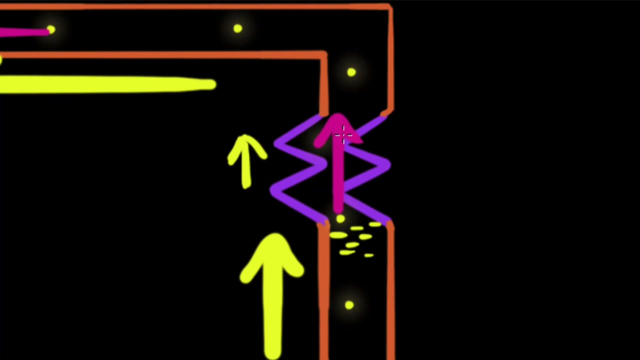 So you have electrons accumulated, which means you have negative charges accumulated. Let's draw that. So here are our negative charges getting accumulated And similarly, what's gonna happen here? you have electrons going out of this point very quickly, but you have less electrons coming into that point. 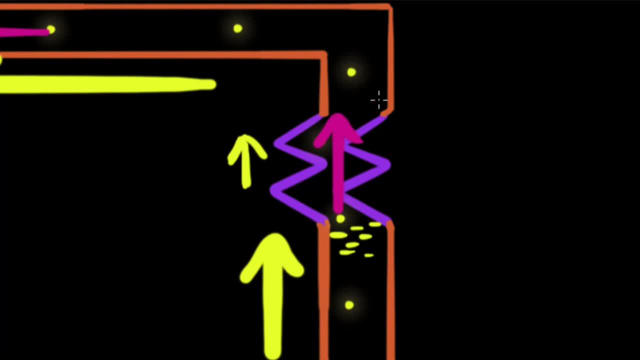 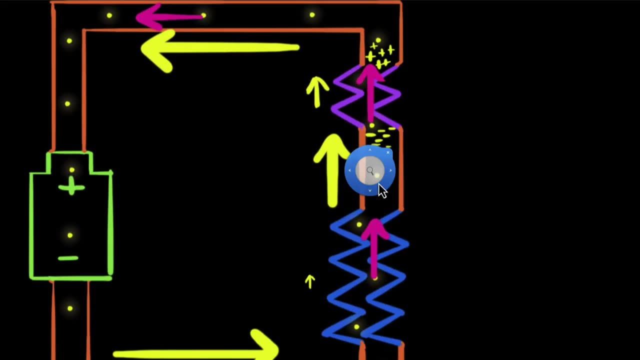 and therefore the opposite effect is going to happen. It will be deficient of electrons and therefore you'll have positive charge on this end. So you have charge accumulation happening at the ends of the resistor. The same thing's gonna happen over here as well. 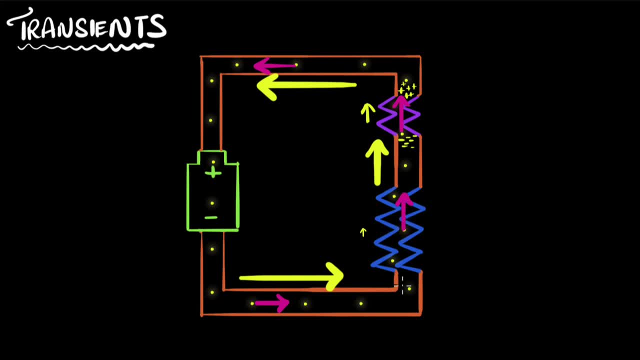 But my question to you is: do you think the charges accumulated over here would be more than what we get over here, Less, or is it gonna be the same? What do you think? Well, because the difference in the current is much higher here than over here. 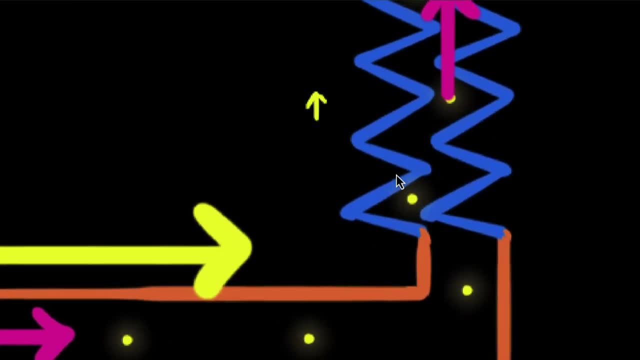 the effect is amplified. So if I look at over here, you have a lot more electrons flowing in per second and a lot less electrons flowing out and therefore you have a lot more charges accumulated, a lot more negative charges being formed, okay, per second. 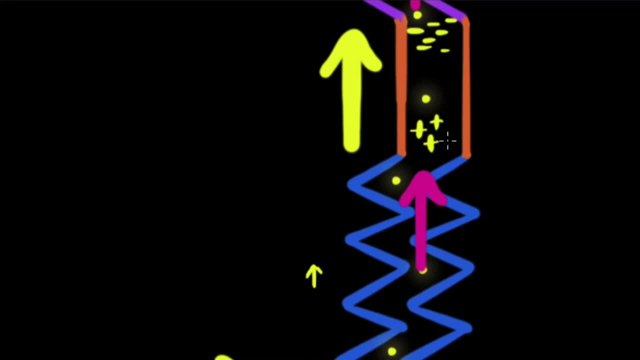 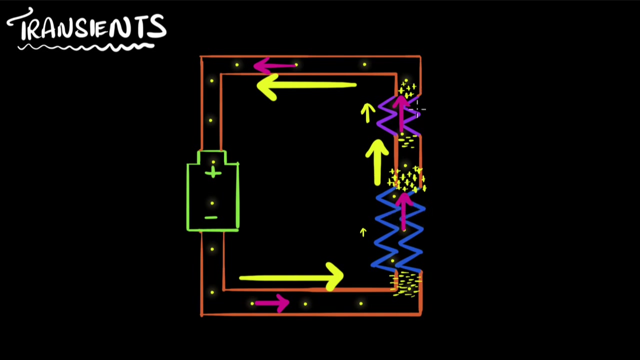 Any given moment in time you'll have a lot more charges accumulated. I'm gonna draw so many so we can clearly see the difference between these two and right at this moment. hopefully it gives you hints of why the voltage across the two resistor. 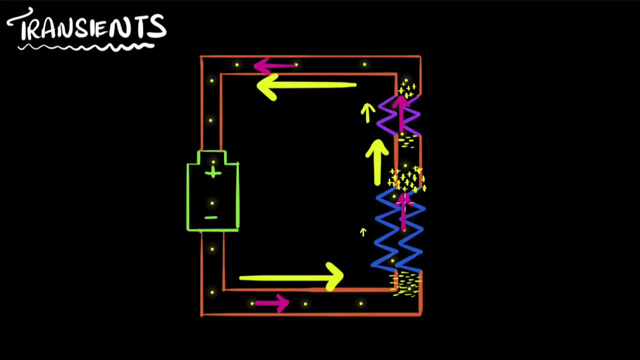 doesn't happen to be the same. You can sort of see why the voltage across the bigger resistor starts becoming more than the voltage across this resistor. Can you see that? But anyways, we're getting ahead of ourselves. It's just a hint. we still haven't solved anything. 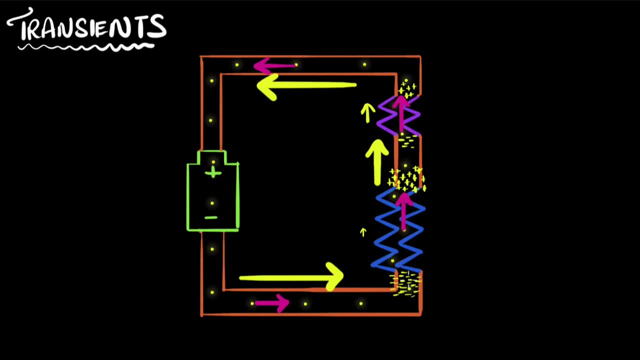 The question now is: what's going to happen because of these accumulated charges? These are gonna have a huge role to play. They're gonna have a very important role in what happens next. What are they gonna do? How are they gonna affect our circuit? 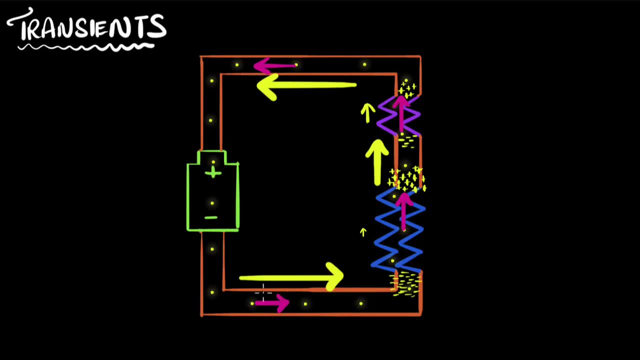 Well see, so far the electrons are experiencing a force, the force only due to the battery right. But now these charges are also going to start influencing these electrons, They're also going to start pulling and pushing on them. 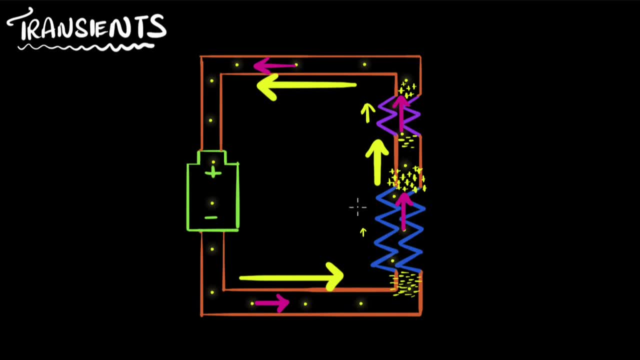 As a result, the forces will change. As a result, the current will start changing. How will it change? Let's look at each section of the wire. If I look at this section of the wire, notice the electrons are running into negative charges. 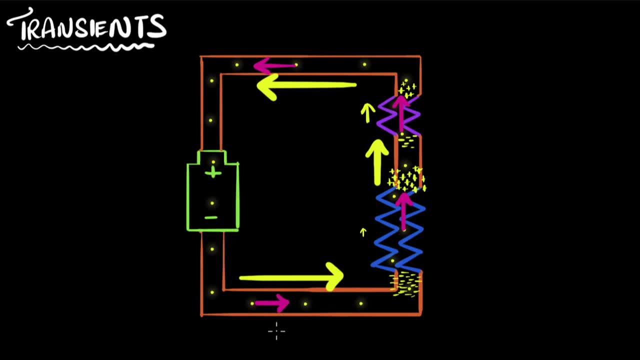 The negative charge is going to repel it. It's gonna push away from it. So what's gonna happen to this force? That is going to be smaller. So this force will be smaller. I'm gonna draw a smaller force. What happens to this one? 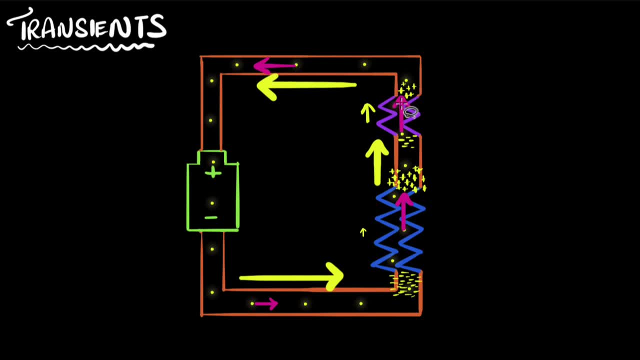 Notice: electrons are moving away from the positive charge. The positive charge is gonna pull it back, Which means again the net force is gonna be smaller. This force is also gonna be smaller, smaller. Same is going to happen over here as well. The forces in this reduce the same. 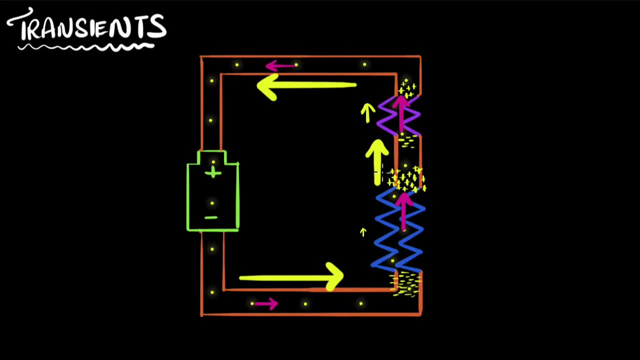 thing happens here. So what happens to these currents? Ooh, this current starts reducing. this current over here starts reducing. I'm going to draw a smaller arrow mark. Let me just write: reduce, reduce, current, reduce, current, reduce. So these currents are going. 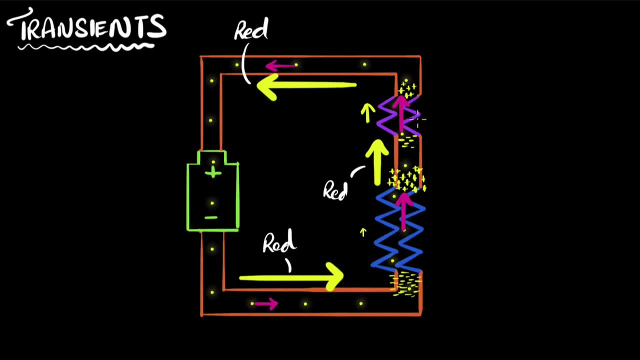 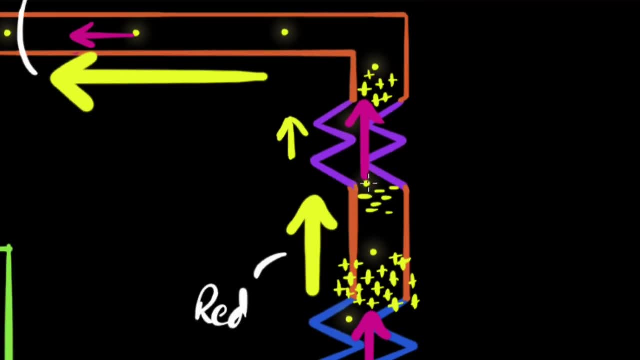 to start reducing What happens to the current in the resistor. Well, for that, let's look at the forces in the resistor. What's going to happen? Well, if I look over here, notice this electron is being pushed away by the negative charge and pulled towards the positive. 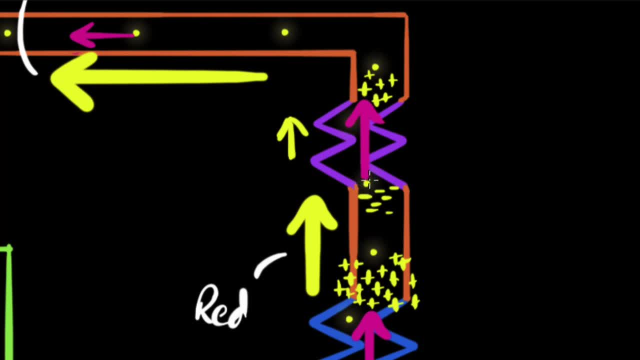 charge, Which means The electron is going to experience more force. The forces are going to add up. Can you see that As a result? as a result, this force is going to be larger. The force on the electrons over here adds up due to the accumulated charges. What's going to happen here? The same effect. 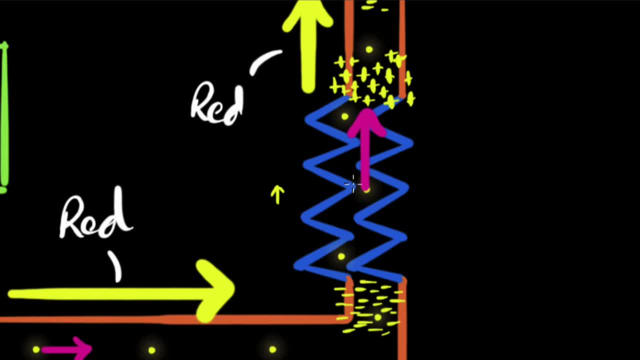 but even more magnified, even more magnified. The electrons are going to be repelled, are going to be attracted, And so the force due to the charges is going to add up to this force and therefore this force. I'm going to draw that over here now so I can draw a big arrow mark, Okay. 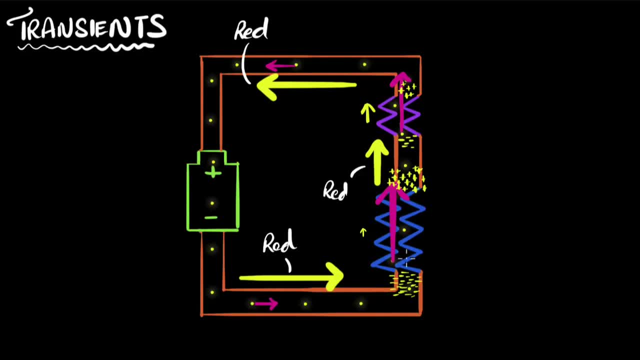 That force is going to get amplified, So it's going to experience even more force inside the resistor And, as a result, what happens to these currents? Ooh, that current is going to increase. So this current is going to increase and this current is going to increase. Can? 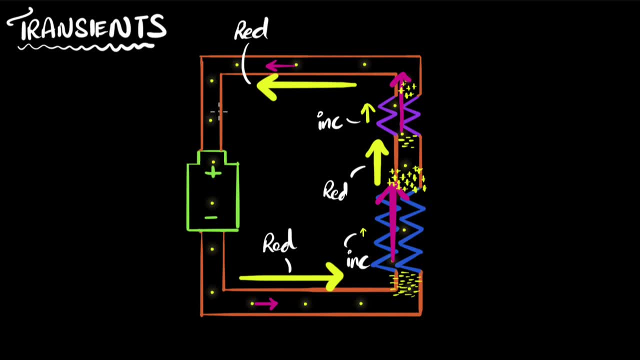 and the stage is set. a couple of things are going to happen. first, you see, the high currents are becoming lower and the low currents are becoming higher. there's a second thing, which is a slightly subtle, even though that's happening, as long as the currents here stay higher than the. 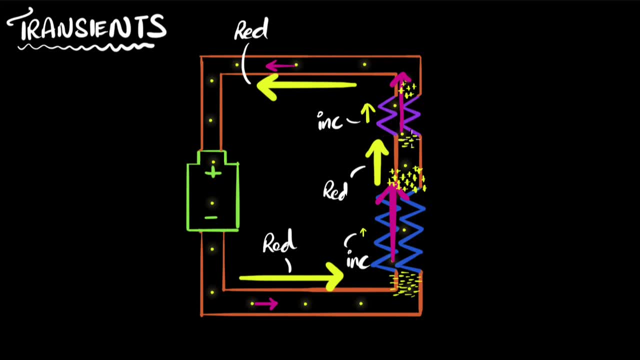 currents. here the charge accumulation continues to happen, which means as time passes by, the effect only gets amplified. the current over here reduces even further, even more quickly. the currents over here is going to increase even more quickly. so not only are these current levels coming closer to each other, but as time passes by, because the charge accumulation, 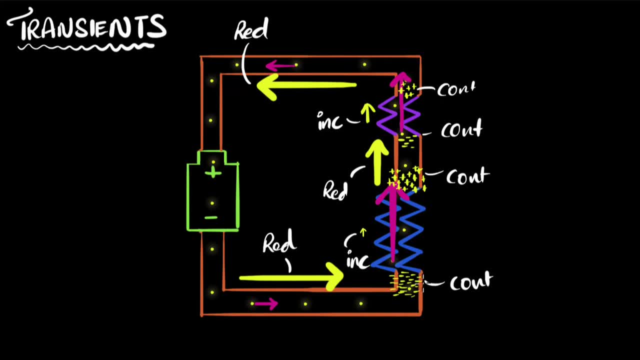 increases. the current levels are coming closer to each other quicker and quicker, and that gives you some insights into why the transients only last for a very small moment. this is happening super fast, in milliseconds. this all happens, and now we can answer our questions. what causes the? 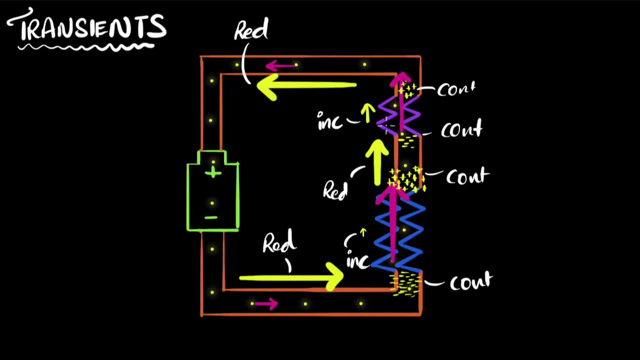 voltage across the resistors in the first place? how does the battery put voltage notice? the battery doesn't put any voltage. it doesn't transfer any voltage at all. the voltage across the resistor is not transferred at all. the voltage across the resistor is not transferred at all. the voltage 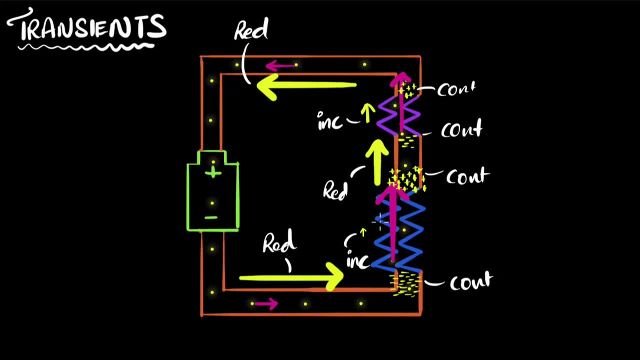 is set up due to the charges accumulated, due to the differences in the current. that's how the voltages are set up over here, and because bigger resistors have more charges accumulated across its ends, because there's more current difference, automatically you end up with more voltage. why? 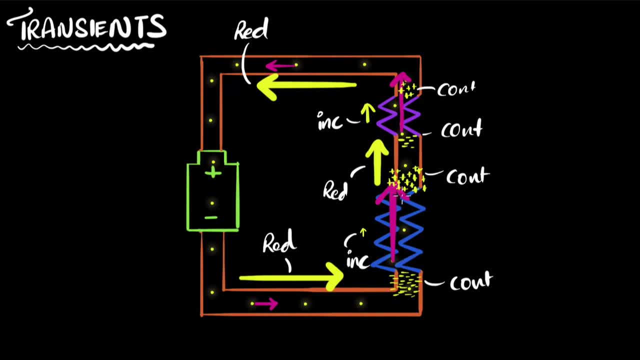 do we say there is more voltage because these accumulate charges are pushing more on the electrons, transferring more energy into the electrons, and therefore we say there is a higher voltage across this resistor, whereas there is lower voltage across the smaller resistor. you see that. do you see how it automatically happens if 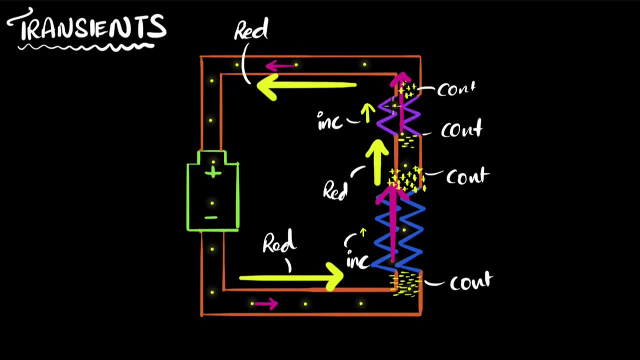 this resistor is, let's say, four times as big as this resistor, the charge accumulated will also be four times as big as this resistor and therefore the push that we'll get over here will be due to. the charges will be four times as much as what we get over here and therefore the voltage across. 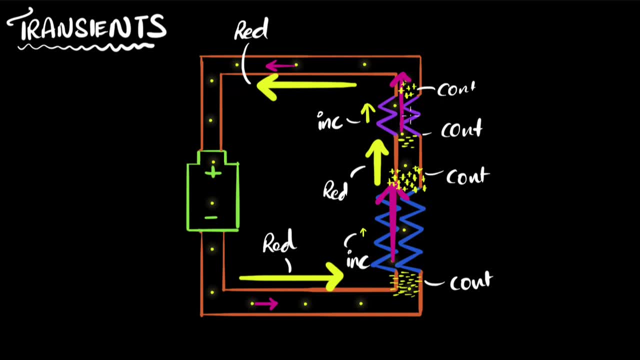 this will also be four times as much as the voltage across over here. that's why the voltage splits. splits in ratio of what the resistances are. okay, so we have voltages that are rising inside the resistor. we have voltage over here four times as much the voltage over here. we have the currents. 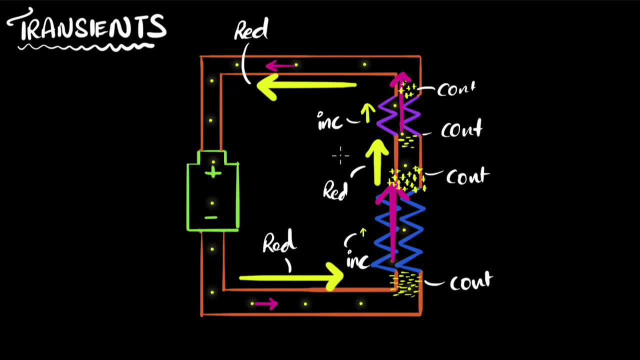 trying to equalize. when is it all going to stop? well, eventually there comes a point when the current here in this section of the wire exactly equals the current in the resistor. why would that happen? because, until that happens, charges will keep on getting accumulated and forcing this current to increase. 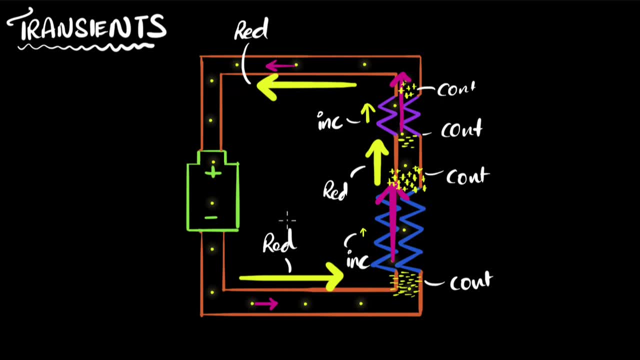 forcing the current to reduce. so eventually that situation must happen. if one thing is reducing and another thing is increasing continuously, eventually, at some point in time they must equalize right. so that moment has arrived. the current now has equalized everywhere. when the current is equalized,